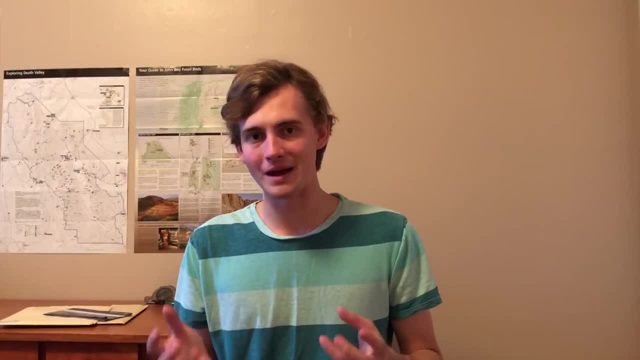 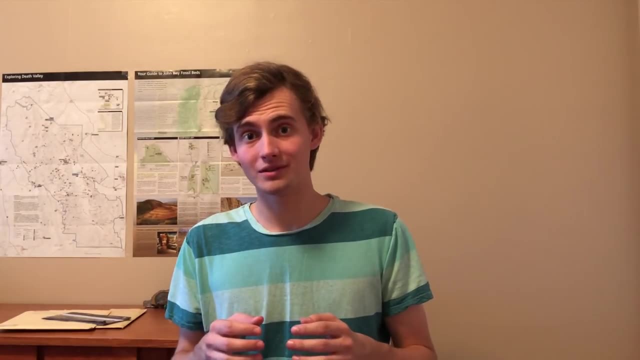 geology in particular. Just about everyone has used a paper roadmap at some point in their life, but there is an entirely different facet to mapmaking that is used to provide data about the world around us. I'm going to use three maps of the same area to give an understanding. 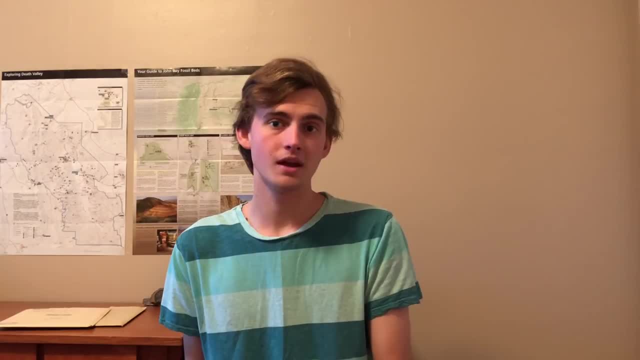 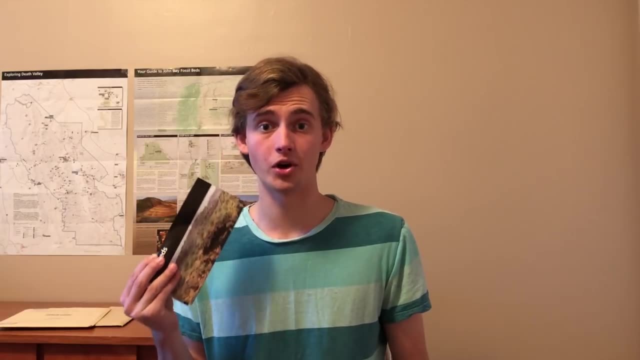 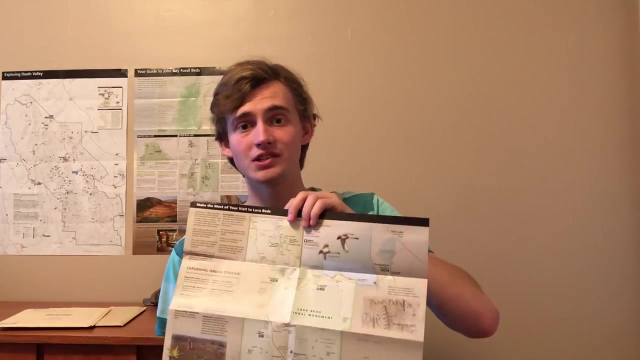 on the similarities and differences between maps. National Park Units in the United States have a standard type of map. This is the map for Lava Beds National Monument in far northern California and it's a very good example of a tourist map. As you can see. it's very easy to read and has lots of information on both sides. 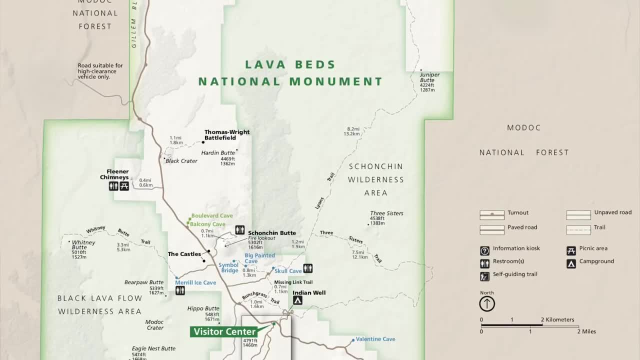 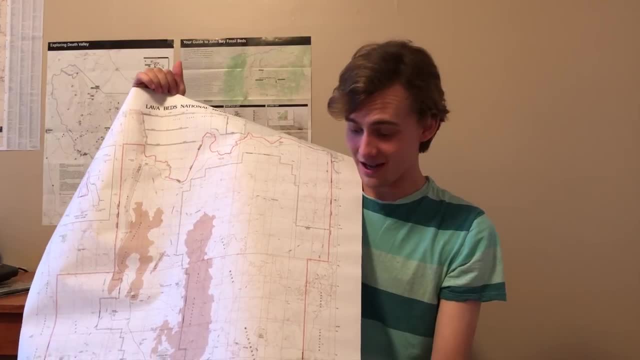 Tourist maps like this usually only show roads, trails and important places to go, such as campgrounds or points of interest. This is a topographic map of the same area- Lava Beds National Monument- and, as you can see already, it gives a lot more. 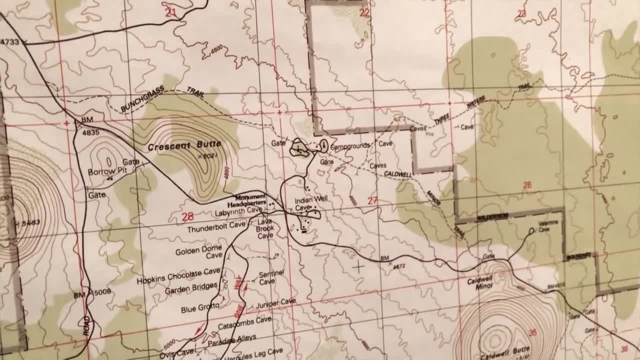 information about the area. This is a map of the same area- Lava Beds National Monument- and, as you can see already, it gives a lot more information about the area And, as you can see, First of all, it's far larger even though it covers roughly the same area, and this allows. 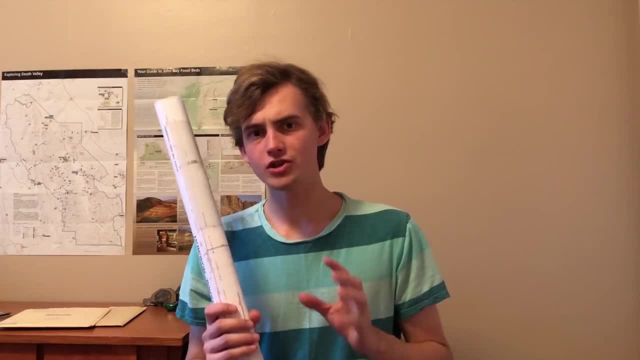 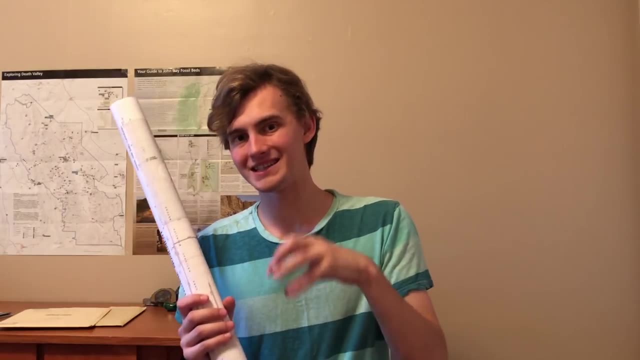 for more detail to be put in the map than it would if it were smaller. A topographic map such as this one primarily gives data about topography in the landscape. Topography is what a landscape looks like, whether it goes uphill or downhill or forms a canyon or a hill. 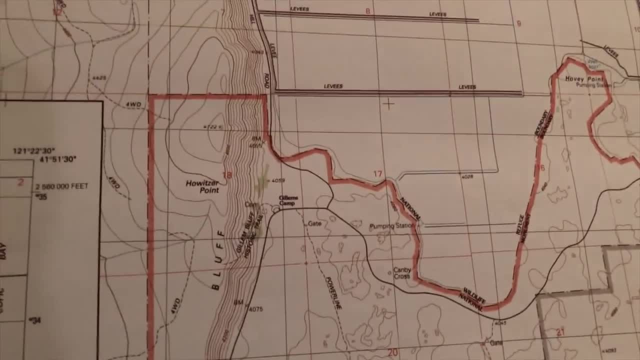 It also gives information about all of the land surfaces, whether it's a road, a parking lot, a building or vegetation or bare rock. It usually gives some kind of indication of what the landscape looks like And, as you can see, it's a map of the same area. 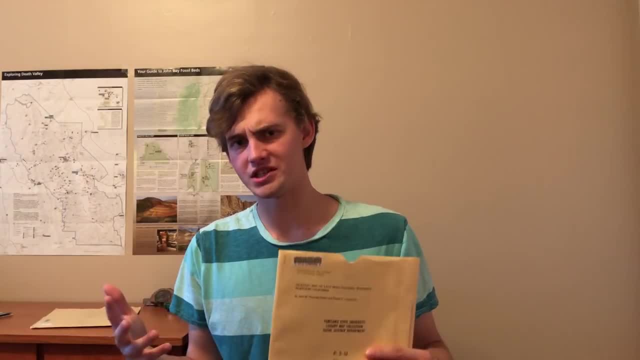 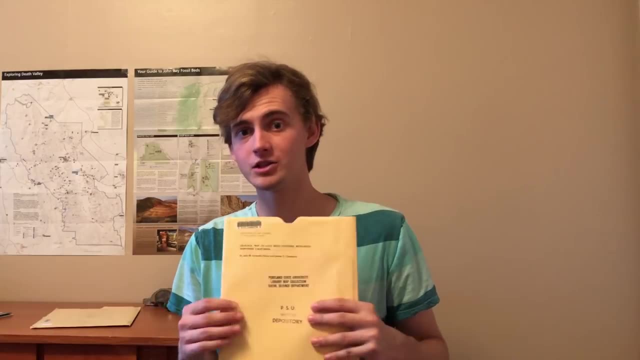 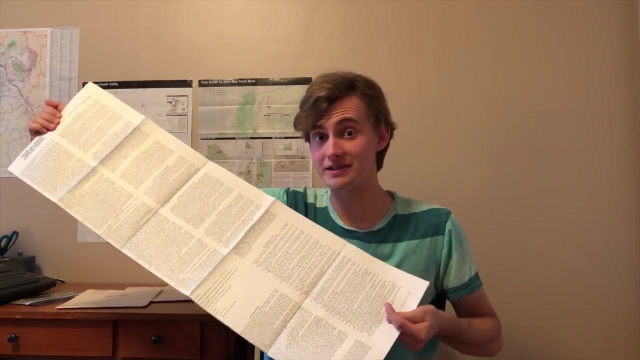 roughly of what it looks like to be on the ground. Geologic and other scientific maps can usually be found at book depositories at research institutions, such as a university library collection. This particular one is from Portland State University's library map collection. Often in geologic maps there's text explaining the different units that are described in the 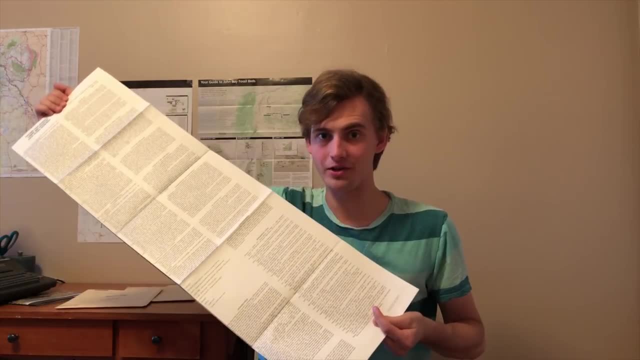 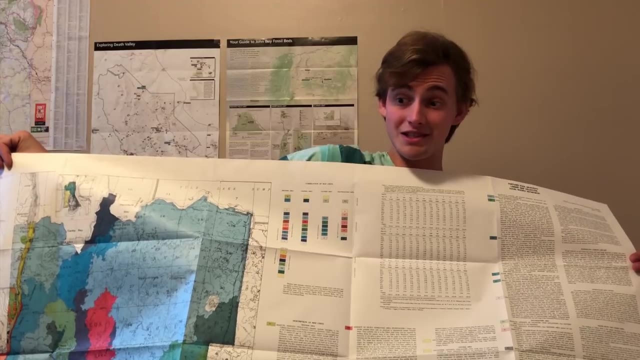 geologic map. Often this is in a book, but sometimes it is printed on the map itself. This is a very large geologic map. The base map for this geologic map of Lava Beds National Monument is the same as the topographic map. What makes the geologic map noticeably different is the amount. 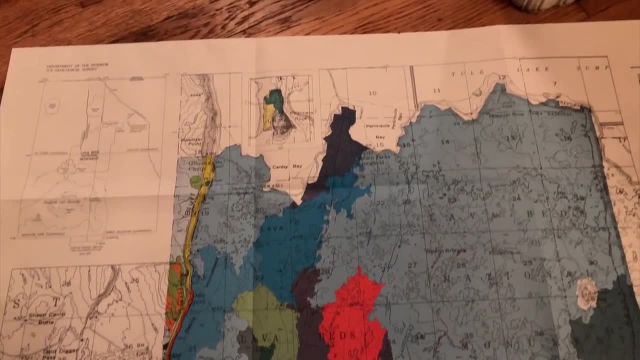 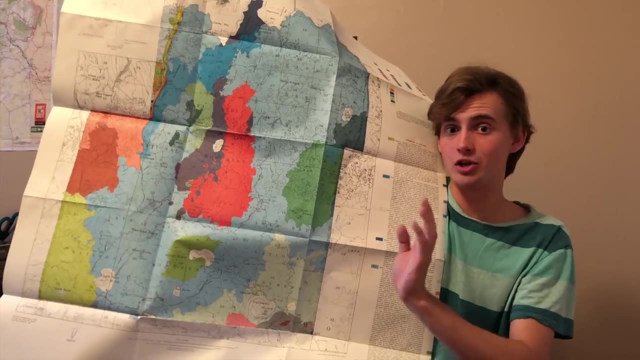 of bright colors. Geologic maps are lots of fun because they have lots of colors. Every color on a geologic map represents a different rock unit. Because Lava Beds National Monument is almost entirely basalt lava flows, all of the rock units on the geologic map are fairly easy.